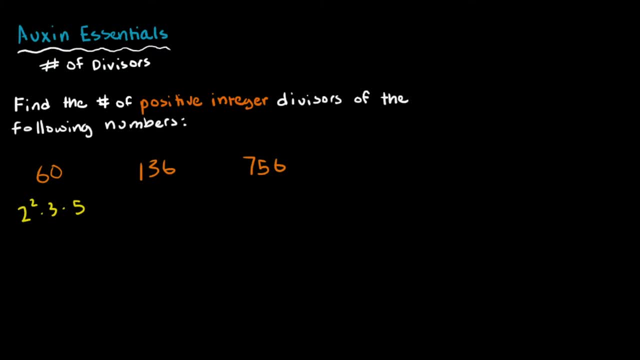 see if we can notice a pattern. So the first, so the first step that we can do, the first step that we can do is we can list out how many ways are there to choose each one of these factors. So we can choose 0 factors of 2 in your, in your factor of 60. You can also choose 1 factor of 2,. 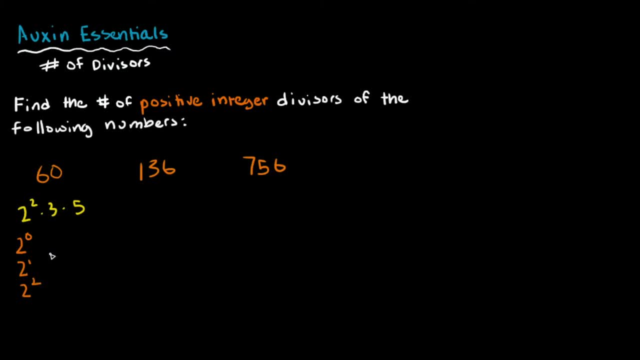 and you can choose 2 factors of 2.. Now, this is 3 ways to choose the number of factors of 2 that you want in your factor of 60. And we can do this similarly for 3 and 5.. Now remember. 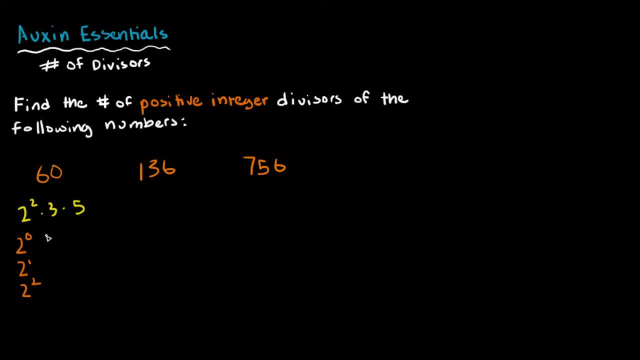 this is actually 3 to the 1,. this is 5 to the 1.. So we can choose a 3 to the 0, and we can choose a 3 to the 1.. Similarly, we can choose a 5 to the 0,. we can choose a 5 to the. 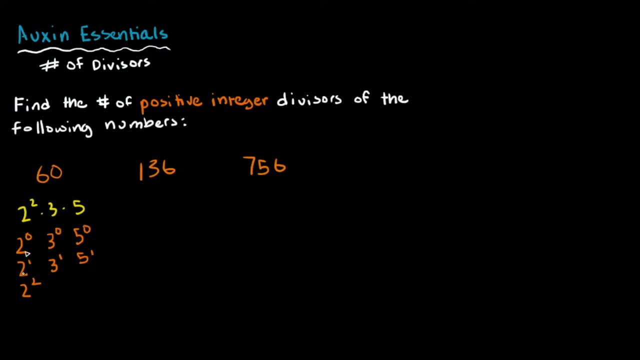 1. And these are all the. if you multiply the number of ways to do each of these, you'll get the total number of combinations. You have 3 ways to do this. You also have 2 ways to do this, and you have 2 ways to do this. So 3 ways to choose. 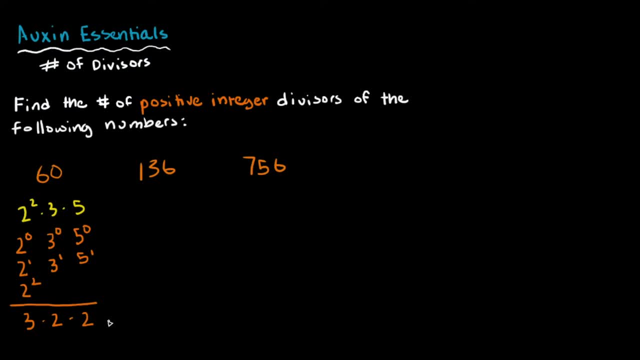 2, 2 ways to choose factors of 3, 2 ways to choose factors of 5.. And this gives you 3 times 2 times 2, which is 12.. And that will actually be our answer for this problem. We have found 12. 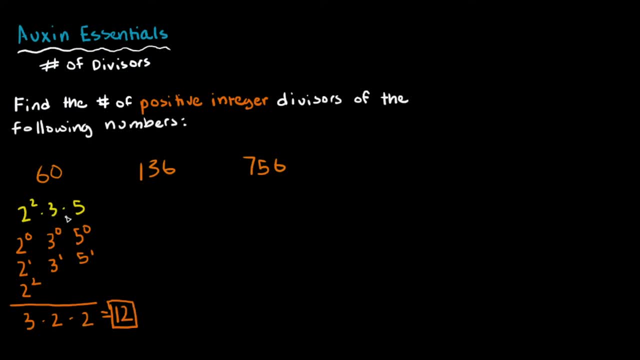 combinations of the ways we can choose a factor from this prime factorization. So let's see if we can notice a pattern from this. Let's see When we have 2, we're actually just having that 1 and 2 here, so that's 2 combinations, But we're also adding the 2 to the 0 here, So let's. 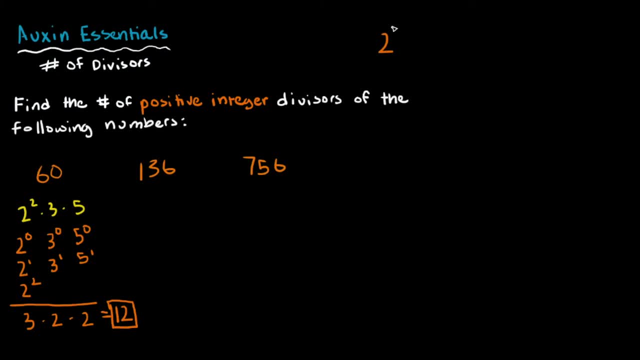 think about this. Well, if you have, if you have a 2 to the n, then you'll include 2 to the 0,, 2 to the 1,, 2 to the 2.. Let's go all the way until 2 to the n. Now this: we know that the numbers from 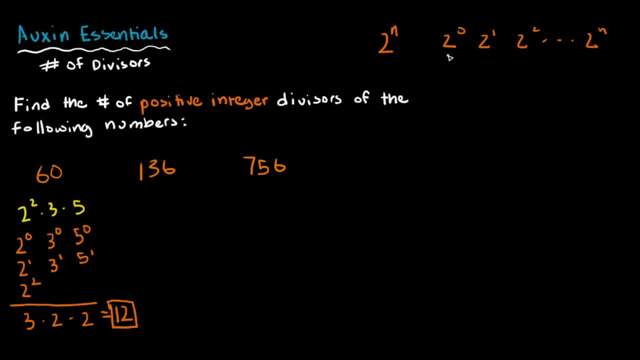 1 to n is n numbers, So we know that this is simply n plus 1 numbers. So what does that mean? What does that suggest? Well, it suggests that these- the way we can figure out this, these 3,, 2, and 2 over here, is: just add 1 to the. 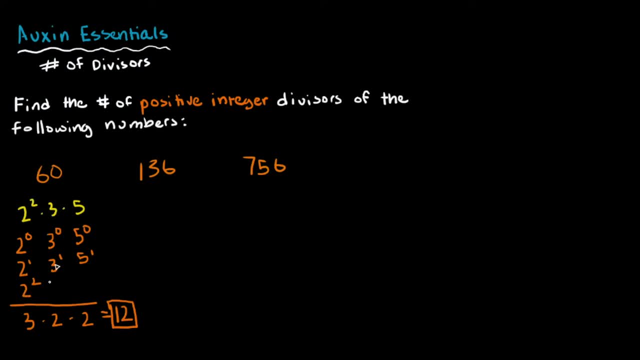 exponent of each of these: 2 plus 1 is 3,. 1 plus 1 is 2,. 1 plus 1 is 2.. So let's see if we can use this newfound knowledge to solve the other problems. 136 is divisible by 4.. So the way we can divide it. 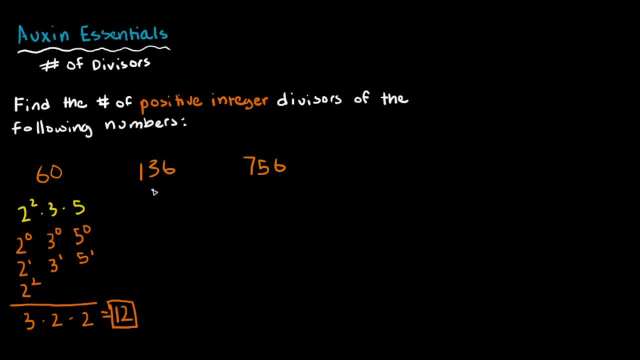 by 4,. well, you just have to divide it by 4.. So you just have to divide it by 4.. So you just have to divide 100 by 4,, which is 25.. Divide 36 by 4,, which is 9.. 25 plus 9 is 34,, which is divisible again by. 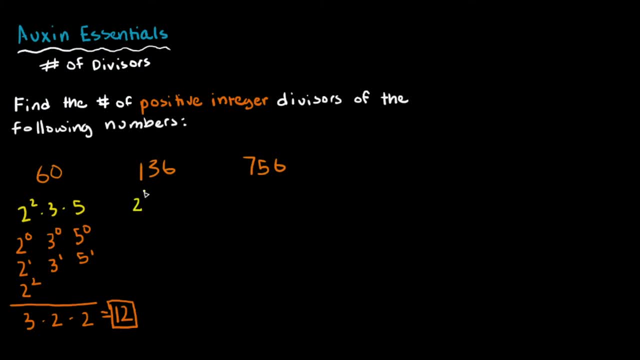 2.. So we know now, so far is we have 3 factors of 2.. And we were we were left with. we were left with 34 when we divided by 4 just now, And we were left with 34, meaning that when we divided by 2, 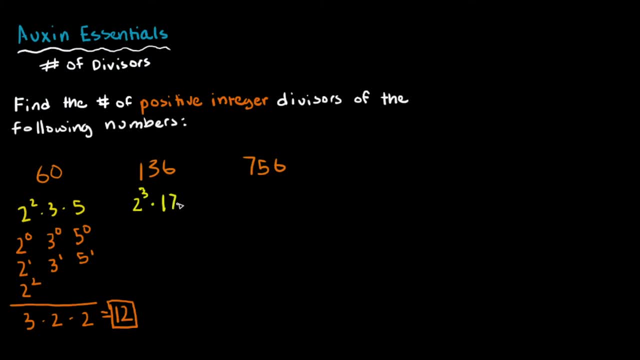 again to get this factor of 8.. We're going to have 17 over here And I want to hit this 1 just to make it clear what we're about to do. So let's see if we can do this without without using listing out all the numbers here. Well, let's see. 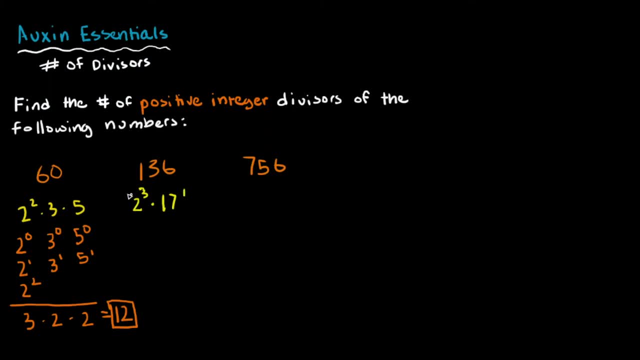 We know that it's n plus 1, the number in the exponent- So let's take n- is equal to 3.. So we have 4 ways to choose a, 4 ways to choose the factors of 2.. Like like, we can choose 2 to the 0,, 2 to the 1,, 2 to the 2,, 2 to the 3.. 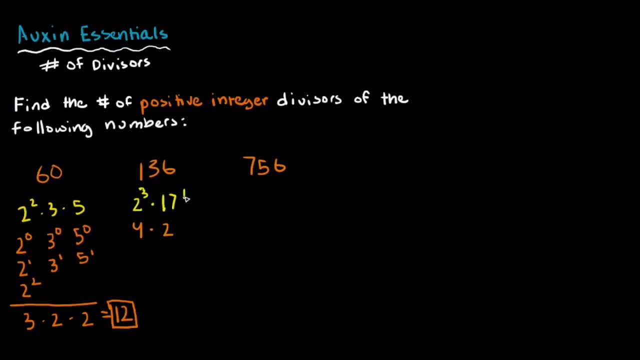 That's 4 ways, And similarly you can choose 2,. you have 2 ways to choose the factors of 17,, 0 or 1.. So we have 3 plus 1,, 1 plus 1, and this is equal to 8,, which is our next answer. 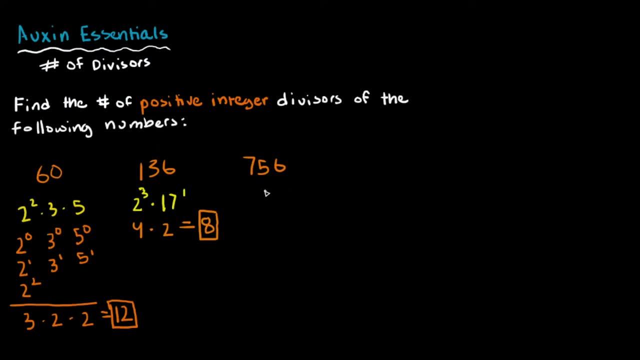 And let's finally look at 756.. So after some factorization, you may realize that, okay, this is divisible by 4, so we have 2 squared. And you may also realize afterward that this is also divisible by 4.. So you know, that's alright.